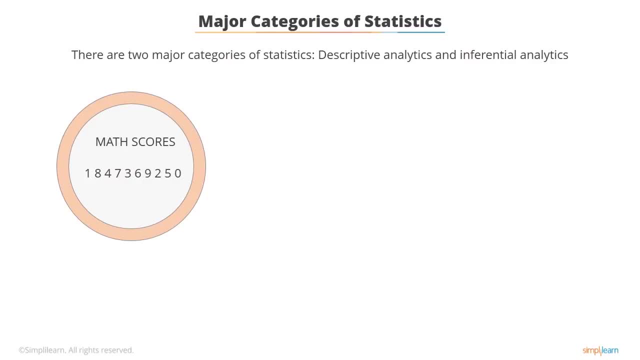 Descriptive analytics helps organize the data and focuses on the main characteristics of the data. It provides a concise summary of the data. You can summarize data numerically or graphically. For example, you can collect all the data about the visitors to your website for a week and summarize the data. 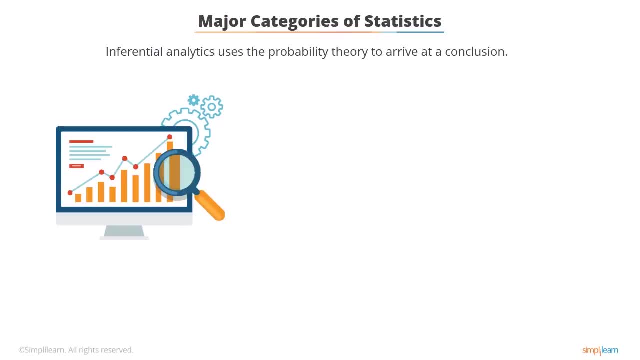 Inferential analytics generalizes the larger data set and applies the probability theory to draw a conclusion. In this approach, a random sample of data is taken from a population to describe and make inferences about the population. Inferential statistics is valuable when it is not convenient or possible to examine each member of an entire population. 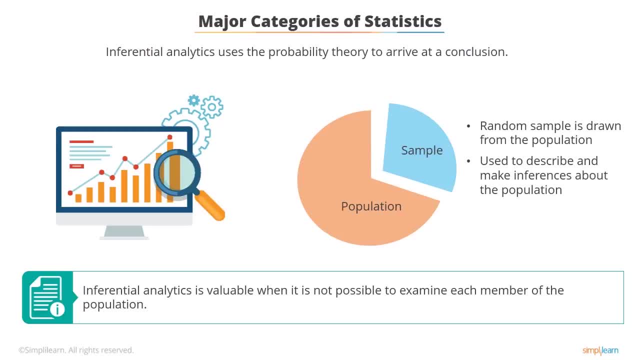 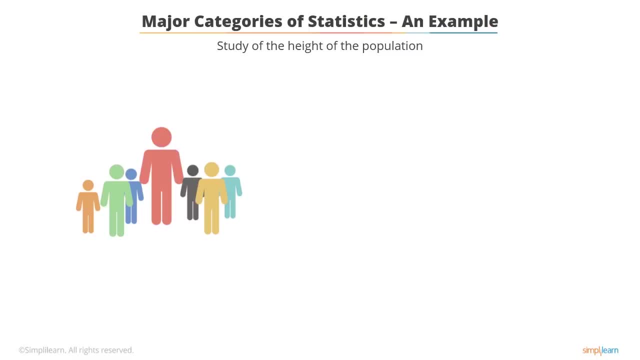 Let's understand both categories better through an example. Suppose you want to study the height of a person in an entire population. You can do this in two ways. Were you to record the height of each person in the population, it would be a tedious process. 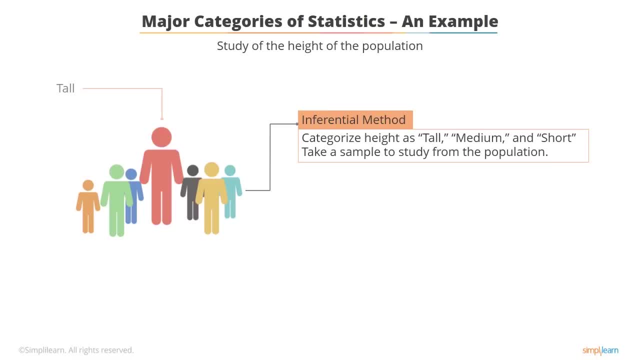 Instead, if you categorize height as tall, medium and small and then take only a sample from the population, this is an inferential analysis. In the descriptive analysis method, you would record the height of every person in the population and then provide the data for the maximum height, minimum height and average height of the population. 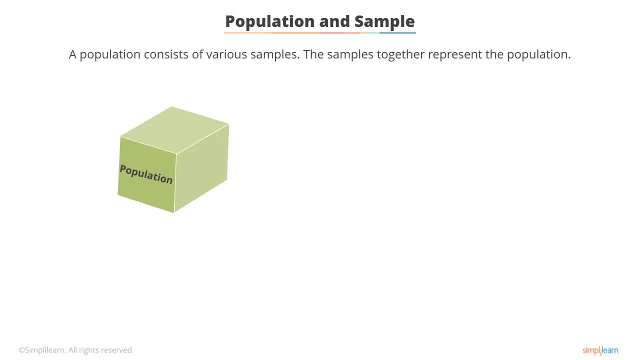 Let's understand population and sample through the visual. Population consists of various samples. A sample is the part or piece drawn from the large population. for statistical analysis, It can be treated as a subset of the population. A sample should be random to help ensure that it has all the characteristics of the population and is also representative of the population. 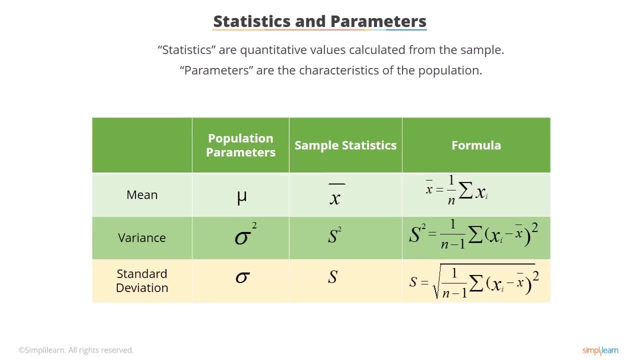 Let's understand the terms statistics and parameters which we'll be using throughout this lesson. Statistics are quantitative values calculated from the sample. Parameters are the characteristics of the population. Suppose you have x0,, x1,, x2, and so on until xn. 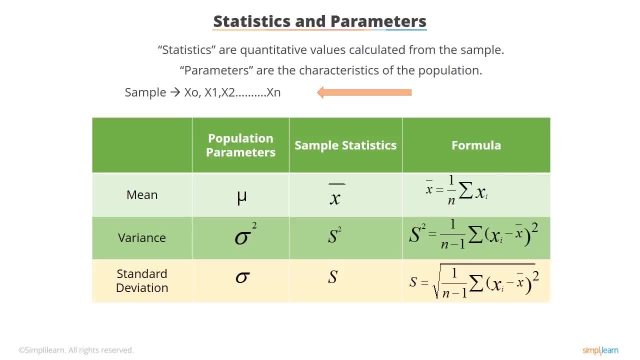 A sample from a population and you want to know some vital information, such as average, most occurring, characteristic and so on. These are calculated using formulas displayed on the screen. Mean is the average, a typical value present in the distribution, and is calculated by summing the values and dividing them by the number of values. 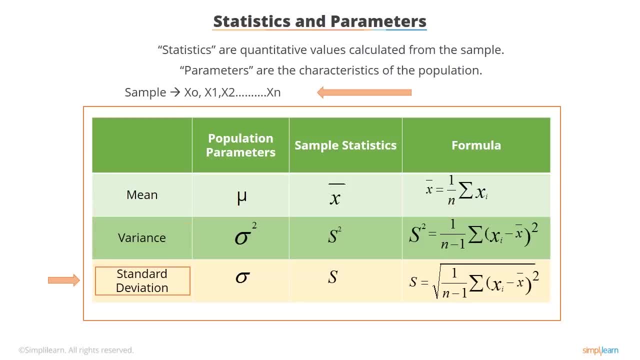 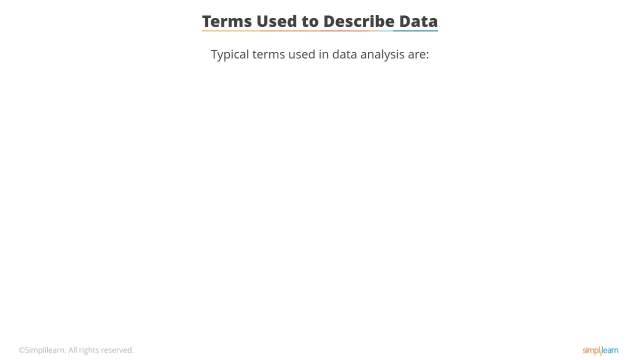 Variance measures. the sample variability Standard deviation explains how spread out the data is from the mean. The greater the standard deviation, the greater the spread in the data. It's measured in the same units as the mean. Certain terms are used in statistical analysis to understand the data and gain insight into it. 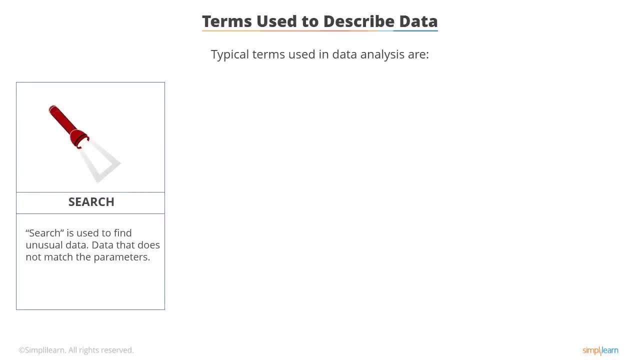 Some of these terms are as follows: Search: Search is typically used to find unusual data. Unusual data refers to those data that doesn't meet the parameters set at the beginning. Inspect: Inspect refers to studying the shape of the data set and determining how spread out it is. 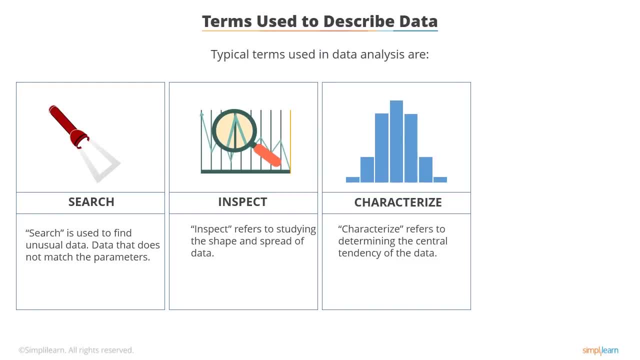 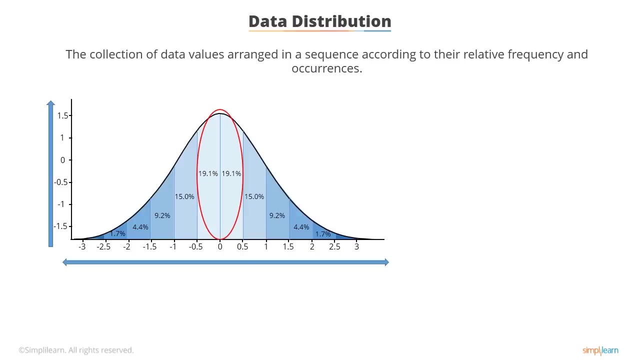 Characterize. Characterize determines the central tendency of the data. Conclusion: Based on the understanding of search, inspect and characterize, we can draw some preliminary or high-level conclusions about the data. Data distribution is the collection of data values that are arranged in order, along with their relative frequency or occurrences. 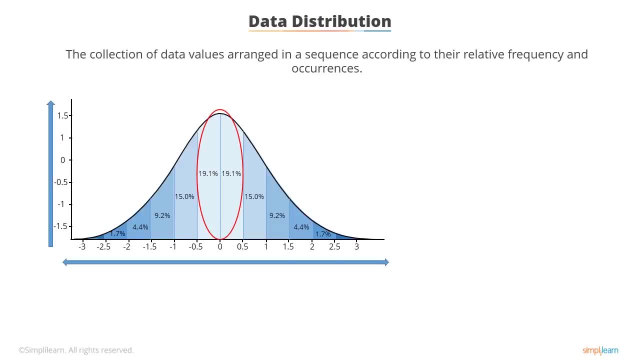 To understand any kind of problem, it's important to describe the data in terms of its spread and shape, using graphical techniques. Range of the data indicates the quantitative values. minimum and maximum Frequency of the data indicates the number of occurrences of any particular data value in the given data set. 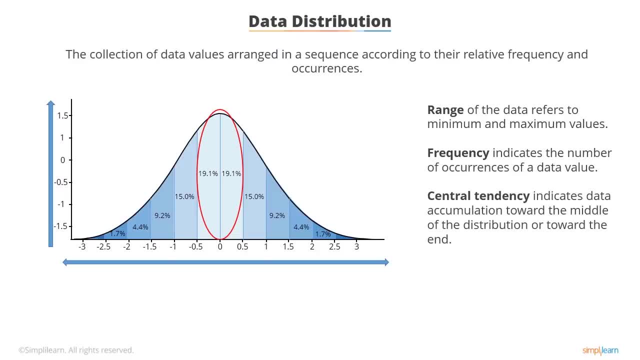 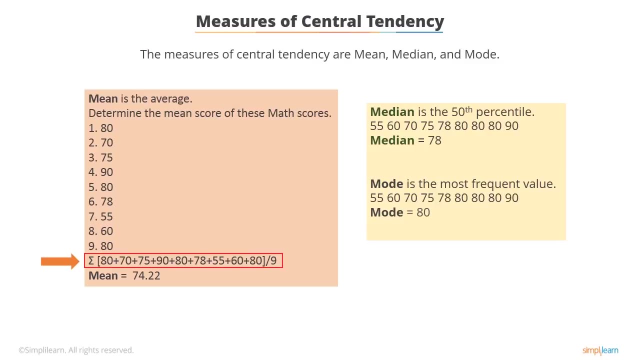 Central tendency indicates whether the data values accumulate in the middle of distribution or toward the end. Following are the measures of central tendency: Mean: The sum of all the values in the data set divided by the number of values. Median The data value right in the middle of the data set, or the 50th percentile. 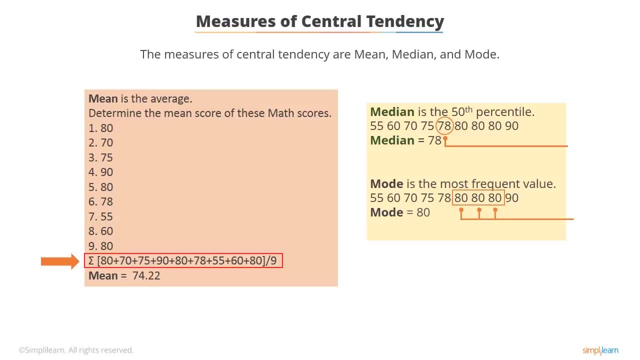 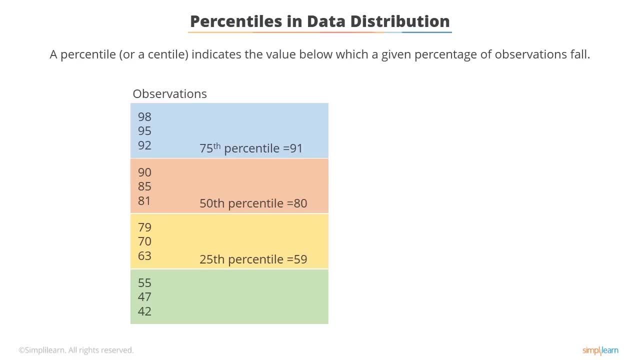 Mode The data value which is the most common or frequent. Let's understand percentile in data distribution. A percentile, or a centile, is a measure used in statistics indicating the value below which a given percentage of observation in a group of observations falls. For example, the 20th percentile is the value or score below which 20% of the observations may be found. 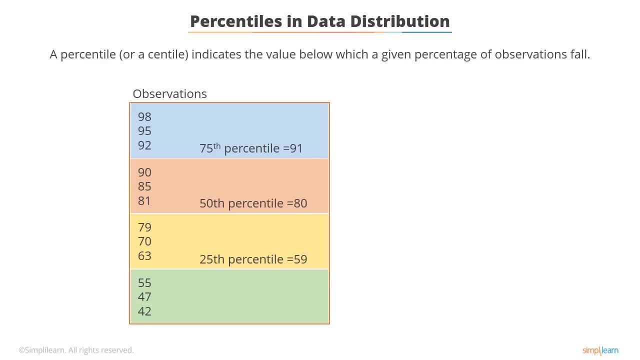 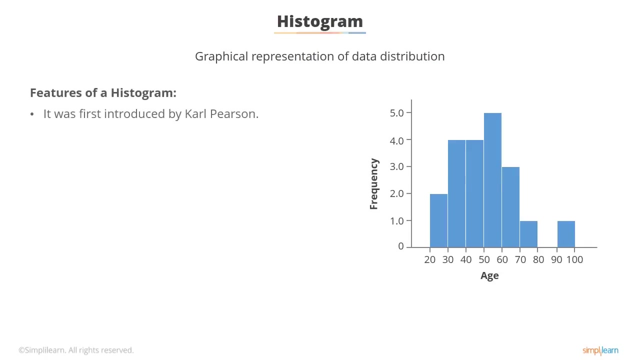 Usually we report percentiles as below: The 25th percentile is called the first quartile. The 50th percentile is called the median or second quartile. The 75th percentile is called the third quartile. Histogram is a graphical representation of data distribution, first introduced by Carl Pearson. 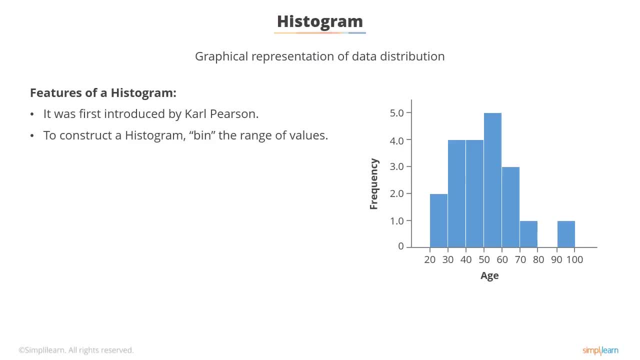 To construct a histogram, the first step is to bend the range of values, That is, divide the entire range of values into a series of intervals and then count how many values fall into each interval. The bends are usually specified as consecutive, non-overlapping intervals of a variable. 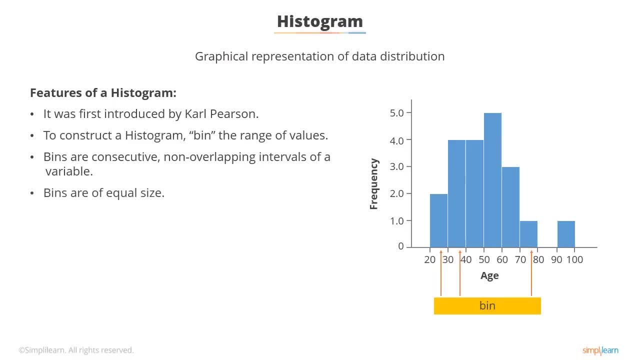 The bends must be adjacent and are usually of equal size. Interval In the graphical representation. each bar represents a group of values, also called bend. The height of the bar represents the frequency of the values in the bend. Histograms help assess the probability distribution of a given variable by depicting the frequencies of the observations occurring in a certain range of values. 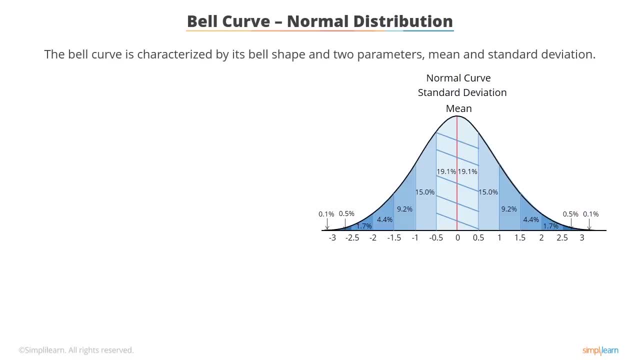 A normal distribution is the most commonly used distribution in statistics. It is characterized by its bell shape and its two parameters: mean and standard deviation. A bell curve or normal distribution is symmetric around the mean. If you draw a line at the center, you'll get the symmetric shapes on both sides. 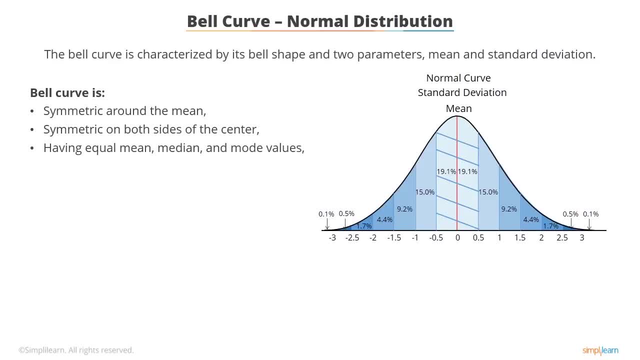 The mean, median and mode of a normal distribution are equal. Normal distributions are denser in the center and less dense in the tails or sides. Normal distributions are denser in the center and less dense in the tails or sides. Normal distributions are defined by two parameters: the mean and the standard deviation. 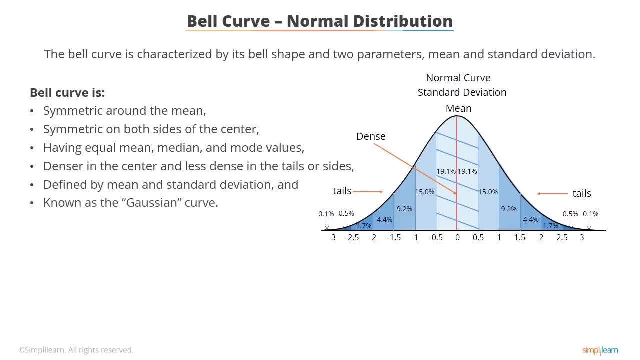 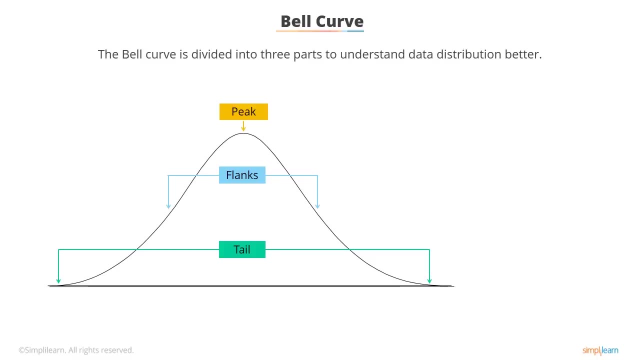 The bell curve is also known as the Gaussian curve. Let's understand the bell curve better. The bell curve is divided into three parts to understand the data distribution better. Peak: It's where most of the observations occur. Generally, The peak is within one standard deviation from the mean. 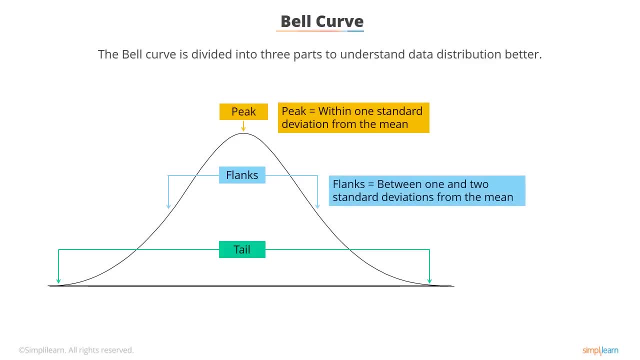 Flanks. They are the areas beyond the peak but between one and two standard deviations from the mean Tails. They refer to the area far from the center of the distribution and considered to be beyond two standard deviations from the mean. Usually, 5% or less data falls under this. 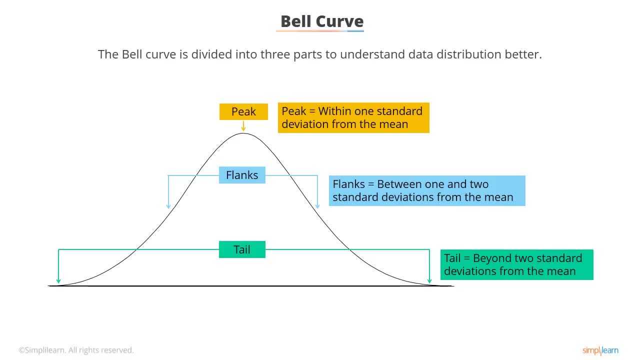 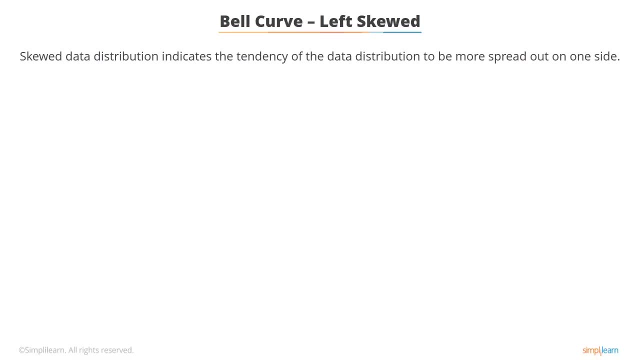 Scales. They refer to those areas above the elementary level. What are the strike points of the trophic usuariis in the individualses A, Motions B, The axis of the top level 3. The group of Ariel of spatula, wall 3.. 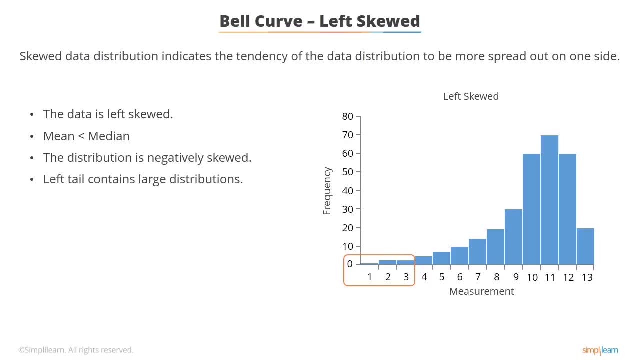 Partial figures: เล 국ний phenomena statement gаго. For example, 혹시 The data is right-skewed or positively skewed, distribution Mean is greater than median. Right tail contains large distributions. Let's now learn about kurtosis, another popular measure of data distribution. 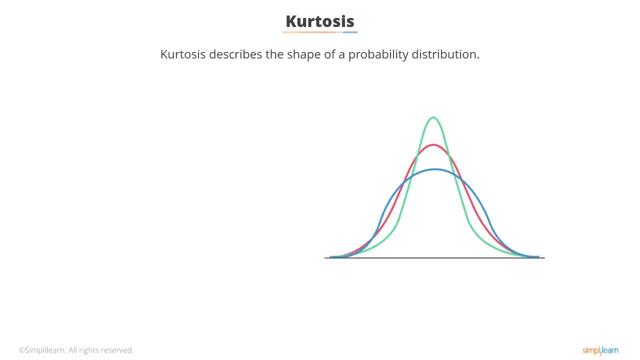 In a similar way to the concept of skewness. kurtosis is a descriptor of the shape of a probability distribution and, just as there are for skewness, there are different ways of quantifying it for a theoretical distribution and corresponding ways of estimating it from a sample of a population. 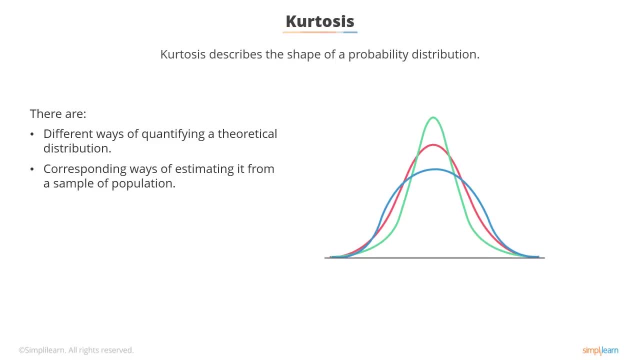 Depending on the particular measure of kurtosis that is used. there are various interpretations of kurtosis. Kurtosis measures the tendency of the data towards the center or towards the tail. Platykurtic is negative statistics or negative kurtosis. 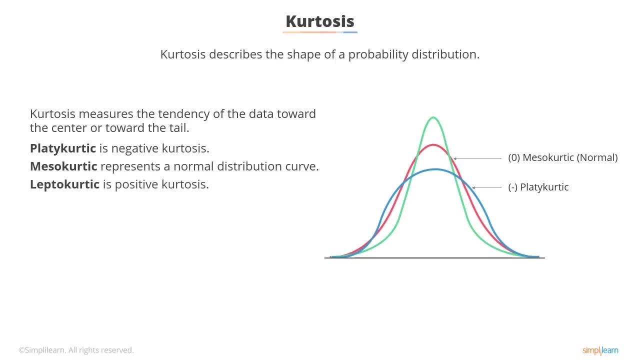 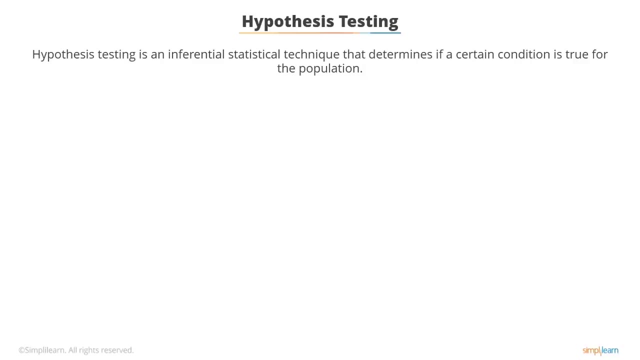 Mesokurtic represents a normal distribution curve. Leptokurtic is positive statistics or positive kurtosis. Hypothesis testing is an inferential statistical technique to determine whether a certain condition is true for the entire population, For example in a manufacturing company. 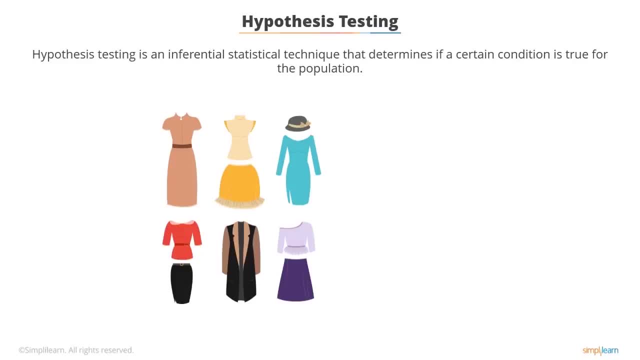 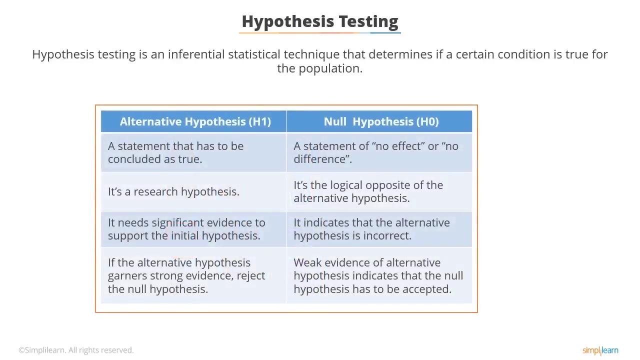 the hypothesis is that every dress manufactured has no defect. A study of each dress manufactured and noting the defects as they occur will prove or disprove the hypothesis that every dress is flawless. A hypothesis test studies two opposing hypotheses about a population. 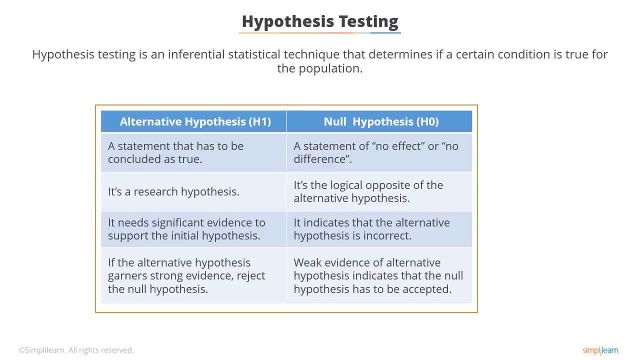 the null hypothesis and the alternative hypothesis. The null hypothesis is the statement that has to be tested. Usually, the null hypothesis is a statement of no effect or no difference. The alternative hypothesis is the statement that has to be concluded as true. To quickly summarize, 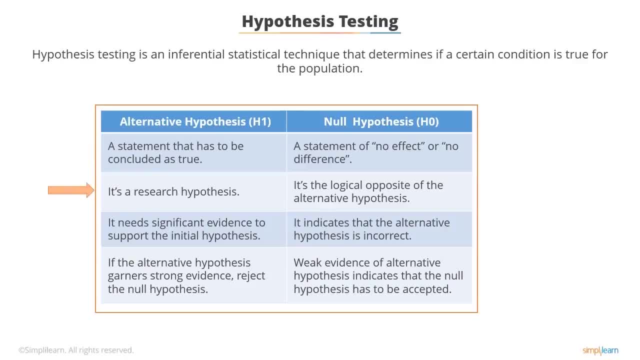 alternative hypothesis. it's a research hypothesis. It needs a significant level of evidence to support the initial hypothesis or assumption. If the alternative hypothesis garners strong evidence, reject the null hypothesis. Null hypothesis: it's the logical opposite of the alternative hypothesis. 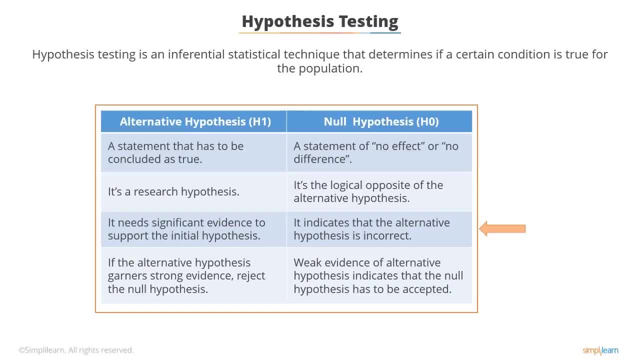 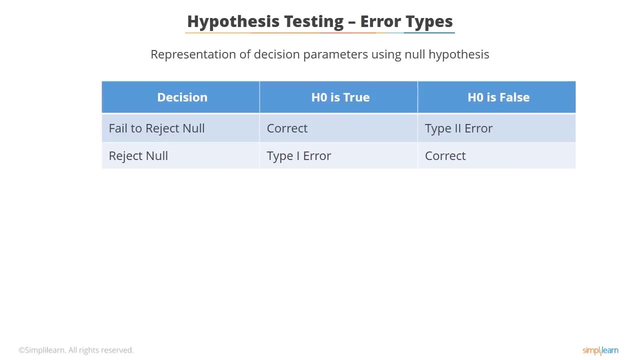 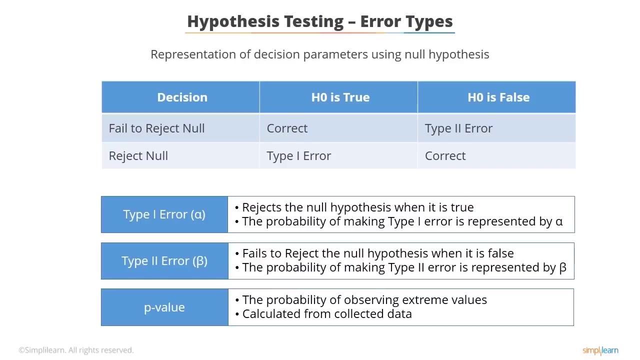 It indicates that the alternative hypothesis is incorrect. Weak evidence of alternative hypothesis indicates that the null hypothesis cannot be rejected. The hypothesis test unusually shows that the null hypothesis has been rejected. The result is difficult to bring to a conclusion. The laboratory Probability value: The probability of observing extreme values or more extreme than the one observed. 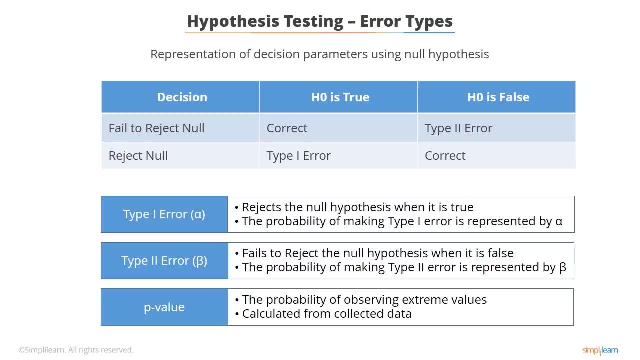 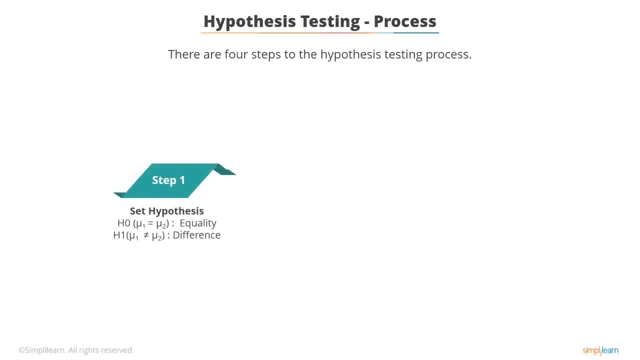 Calculated from collected data. Let's understand the process of hypothesis testing. The first step is to set the hypothesis. The hypothesis could be null or alternative. The null hypothesis, or H0, states that a population parameter is equal to a value. 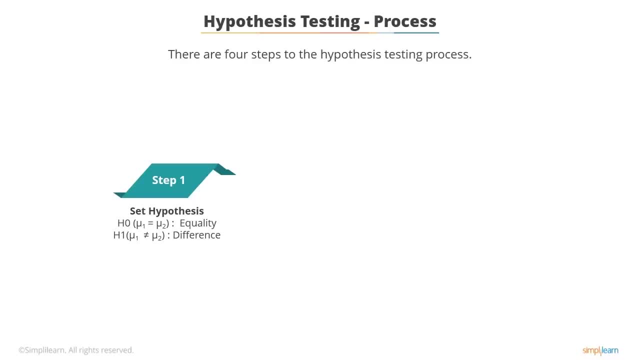 The alternative hypothesis, or H1, states that the population parameter is different than the value of the population parameter in the null hypothesis. The alternative hypothesis is what is believed to be true or is to be proven true. The next step is to set alpha or choose the significant level for the population. 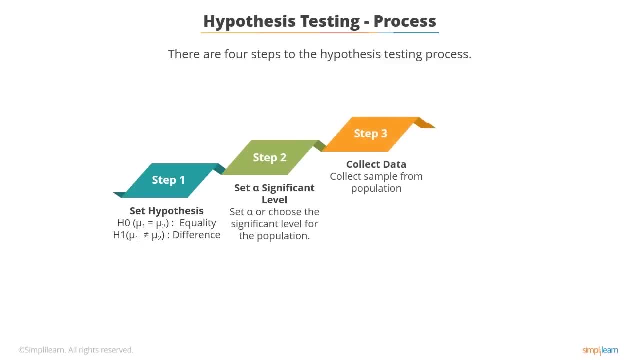 The third step is to set the alpha or choose the significant level for the population. step is to collect the sample from the population, which represents the characteristics of the population. The final step is to compare the p-value and alpha. You reject the null hypothesis. 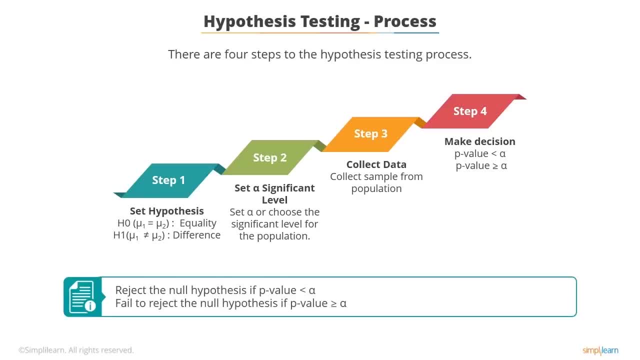 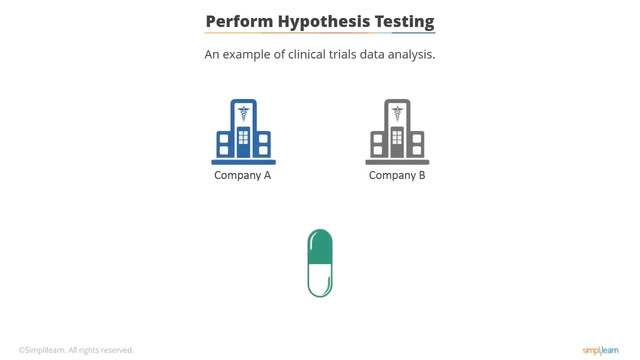 if p-value is less than alpha and fail to reject the null hypothesis if p-value is greater than or equal to alpha. This example shows how clinical trials can be analyzed. Suppose a pharmaceutical company wants to compare a medicine it manufactures with that of a competitor's. 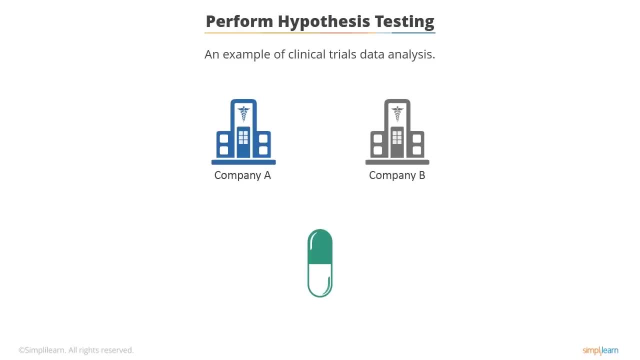 medicine, Then hypothesis testing can be the method it adopts. The null hypothesis would be that both the medicines are equally effective. The alternative hypothesis would be that the two medicines are not equally effective. There are three types of data on which you can perform hypothesis testing. Continuous data: Evaluate the mean. 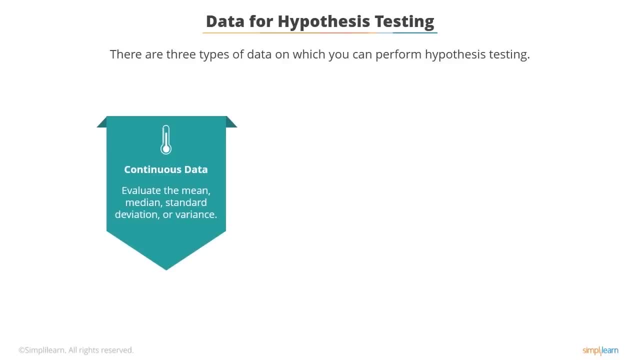 median standard, deviation or variance. If you take the same example, to test the efficacy of medicine, take the temperature of every person in the sample after three hours of administering the medicine. This would be referred to as continuous data, Binomial data. Evaluate the 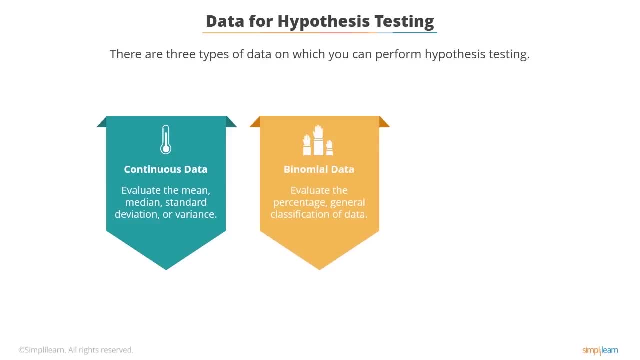 percentage. general classification of data. When data is divided into two categories, you obtain binomial data. If the population were asked if their fever had subsided and the answers could be yes or no, then the percentage who said yes should match the null hypothesis. 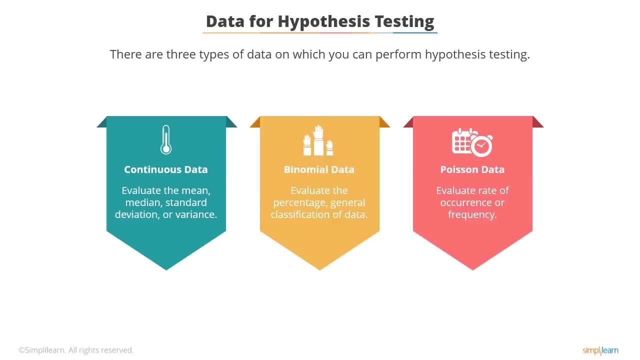 Poison data Evaluate rate of occurrence of frequency If the sample is asked about how many times in a month they use the medicine, and the rate of frequency is recorded and is then compared to the null hypothesis, where the rate should be less than a certain number. 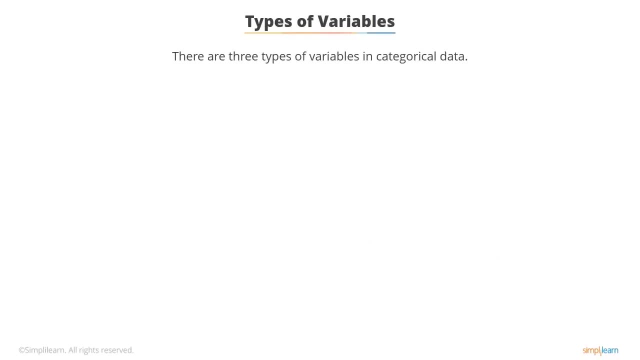 Let's understand the different types of variables to analyze categorical data. Nominal variables have values with no logical ordering. They are independent of each other and the sequence does not matter. For example, in a restaurant you can order burgers, soda and coffee in any order. Ordinal variables have values in logical order. However. 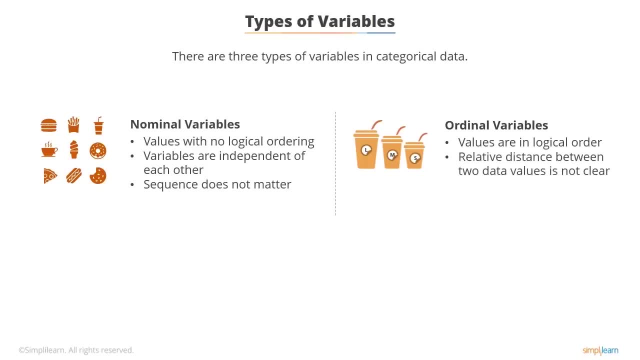 the relative distance between the two data values is not clear. For example, large, medium and small coffee sizes. Association indicates that two variables are associated or independent of each other. For example, in the first data set, weather does not affect the train schedule, but in the 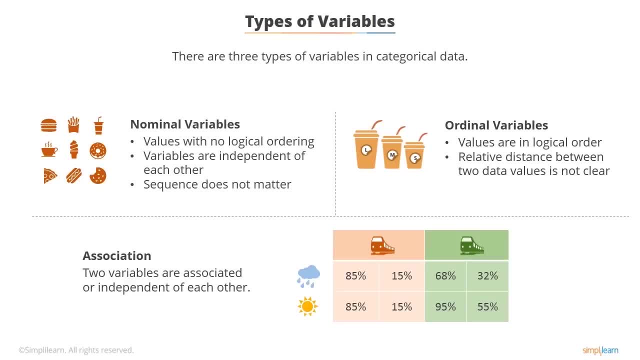 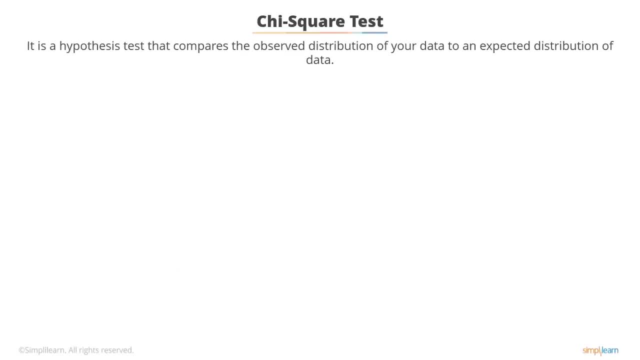 second data set. it does Variables have dependencies and one changes if the other changes. Chi-square test is a hypothesis test that compares the observation distribution of your data to an expected distribution of data. The test is applied usually when there are two categorical variables from a single population. 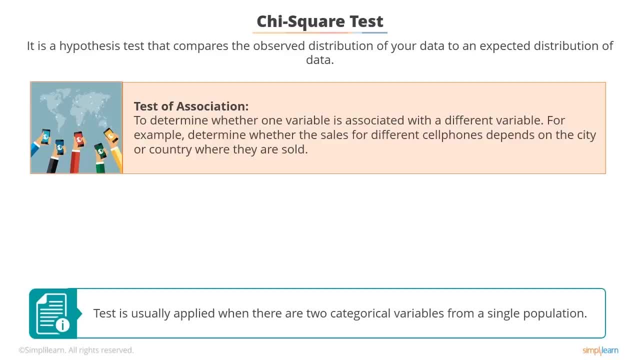 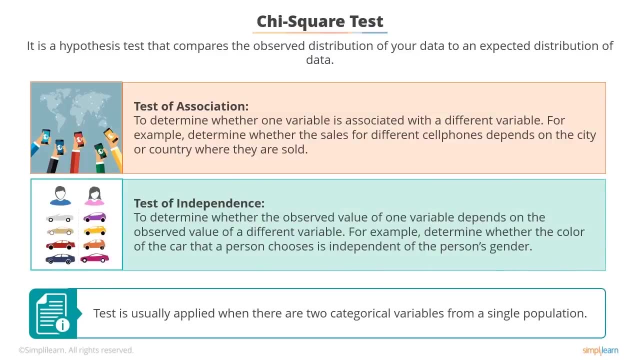 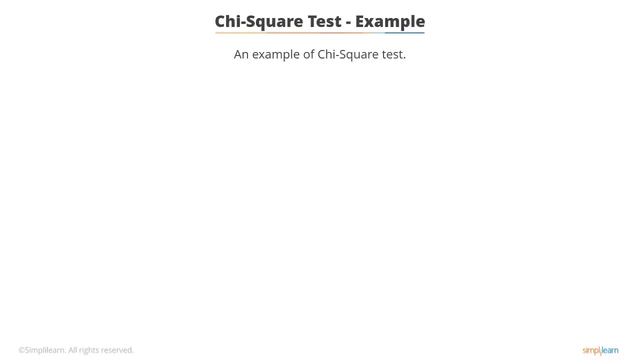 It's used to determine whether there is a significant association between the two variables. Chi-square test is used to test the independence or association between categorical variables. Determine whether a statistical model fits the data adequately. Let's understand the chi-square test through an example. 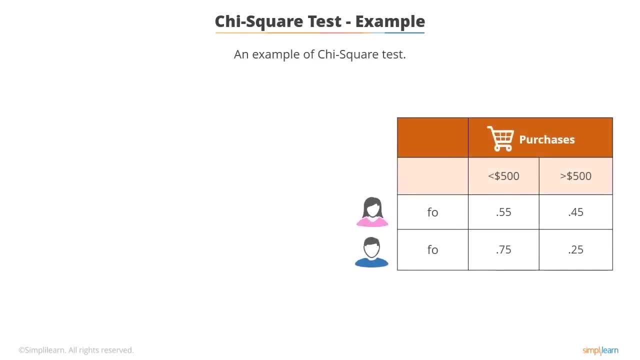 We have a data set of male purchasers and female purchasers. Let's assess whether probability of females purchasing items of $500 or more- or 0.45, is significantly different from the probability of males purchasing items of $500 or more, or 0.25. 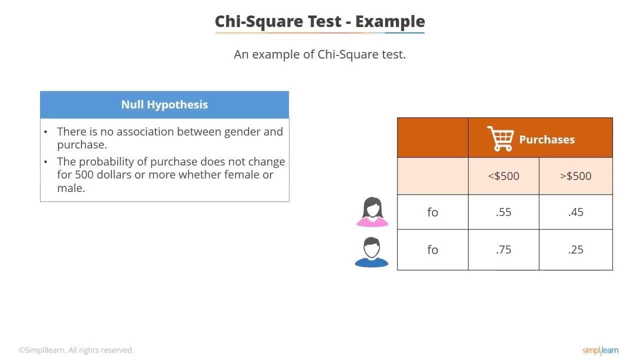 Null hypothesis: There is no association between gender and purchase. The probability of purchase does not change for $500 or more, whether female or male. Alternative hypothesis: There is association between gender and purchase. The probability of purchase over $500 is different for female and male. 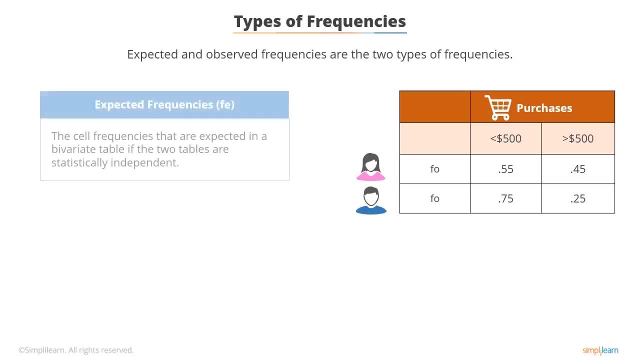 Let's look at the types of frequencies. Expected frequencies or Fe- The cell frequencies that are expected in a bivariate table, if the two tables are statistically independent. Observed frequencies or Fo. There is association between gender and purchase. The probability of purchase behavior over $500 is different for female and male. 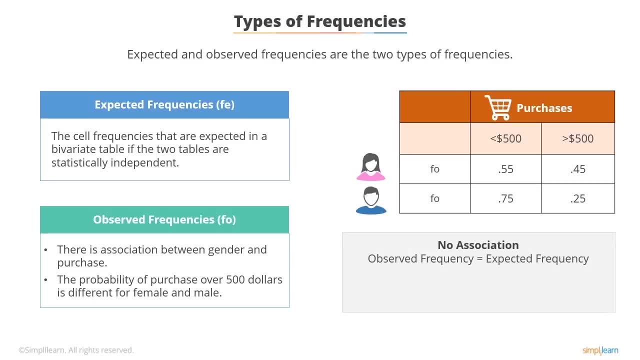 If there is no association between gender and purchase, then the observed frequency would be equal to the expected frequency. If there was an association between gender and purchase behavior, then the observed frequency will not be equal to the expected frequency. The formula for calculating them using chi-square method is shown here. 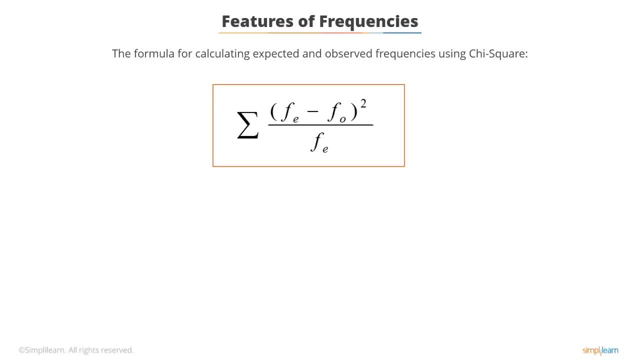 Chi-square is calculated using the formula shown on the screen. Chi-square is the sum of the squared difference between the observed frequency and the expected frequency data, or the deviation divided by the expected frequency data. in all possible categories, Expected and observed frequencies require no assumption of the underlying population. 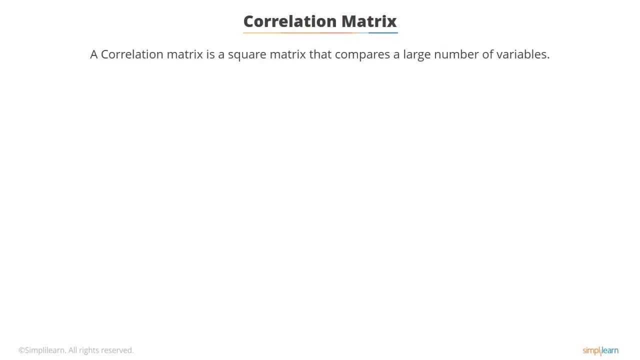 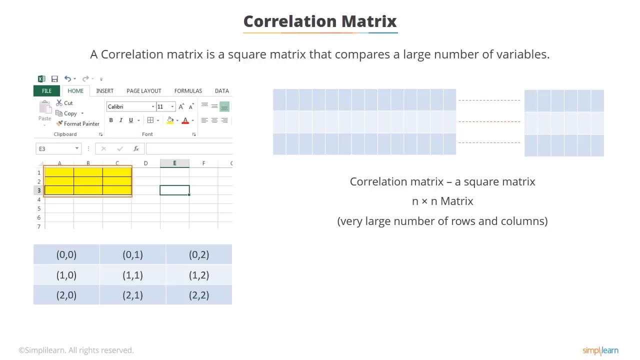 Both the frequencies demand random sampling. Let's understand the correlation matrix. A simple matrix can be visualized as an Excel document with three rows and three columns. A correlation matrix is always a square matrix, That is, it has the same number of rows and columns but it's a larger set. 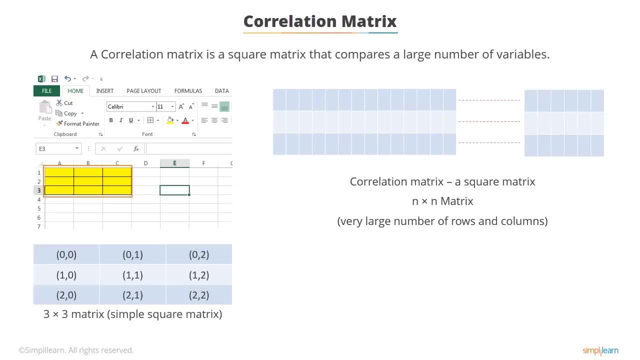 A correlation matrix is expressed in the form of an Xn matrix. When we compare n variables, the covariance is calculated by getting the sample variance between the variables in question. A correlation coefficient measures the extent to which two variables tend to change together. The coefficient describes both the strength and the direction of the relationship. 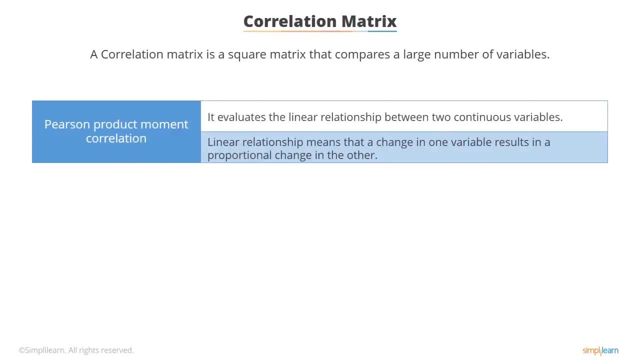 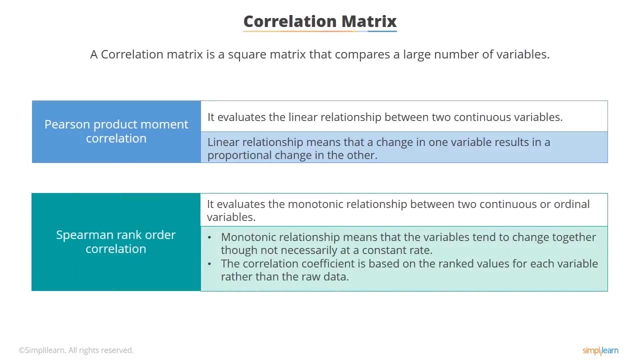 Pearson product moment correlation. The Pearson correlation evaluates the linear relationship between two continuous variables. A relationship is linear when a change in one variable is associated with a proportional change in the other variable. Spearman rank-order correlation, Also called Spearman's row. the Spearman correlation evaluates the monotonic relationship between two continuous or ordinal variables. 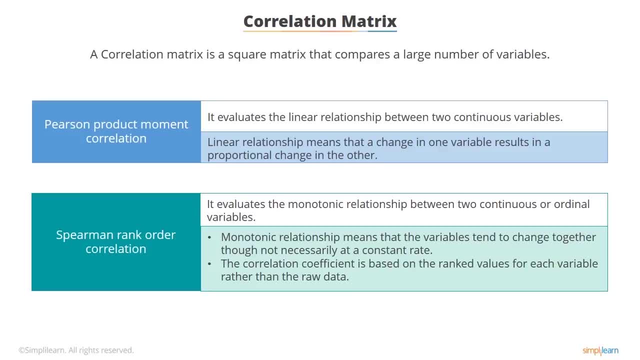 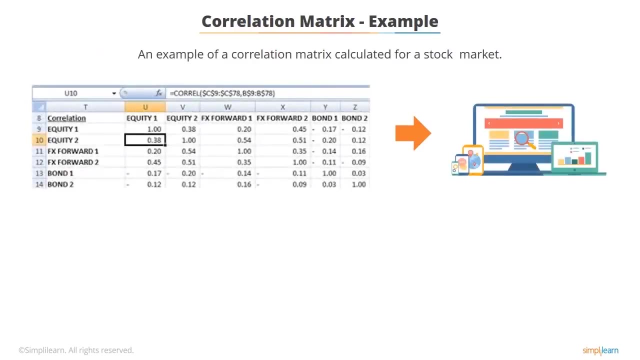 In a monotonic relationship, the variables tend to change together, though not necessarily at a constant rate. The Spearman correlation coefficient is based on the ranked values for each variable rather than the raw data. Here is the example of a correlation matrix calculated for the stock market. 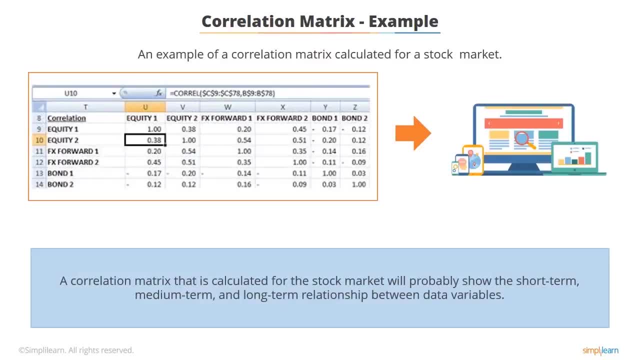 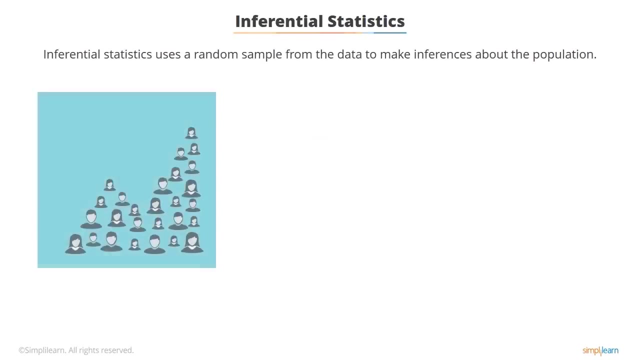 We can choose the data variables and calculate the correlation matrix to demonstrate the short, medium and long-term relationships between them. Now you can see why a correlation matrix would prove useful for traders. We already know that inferential statistics uses a random sample from the data. 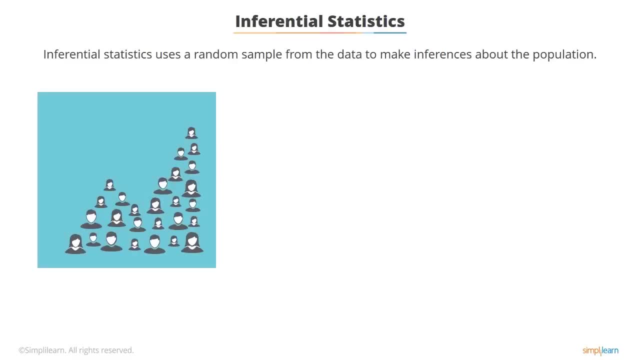 to make inferences about the population. This is a valuable method when each and every member of the population cannot be studied. Inferential statistics can be used only under the following conditions: You have a complete list of the members of the population. You draw a random sample from this population. 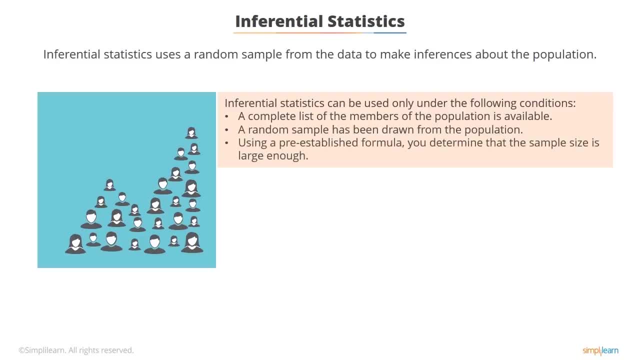 Using a pre-established formula, you determine that your sample size is large enough. Inferential statistics can be used even if your data does not meet these criteria. Inferential statistics can help determine the strength of the relationship with your sample If it's very difficult to obtain a population list and or draw a random sample. 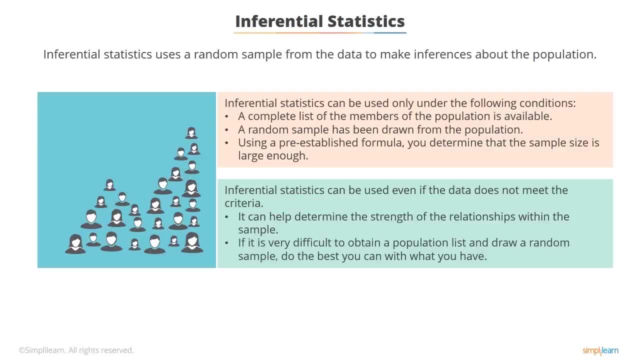 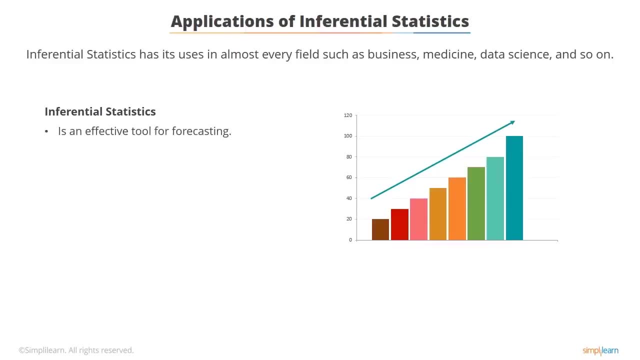 then you do the best you can with what you have. Inferential statistics is an effective forecasting tool widely used in businesses. For example, companies use it to predict their finances for future quarters. Using current data, future patterns can be inferred. Let's now quickly recap what we've learned in the lesson. 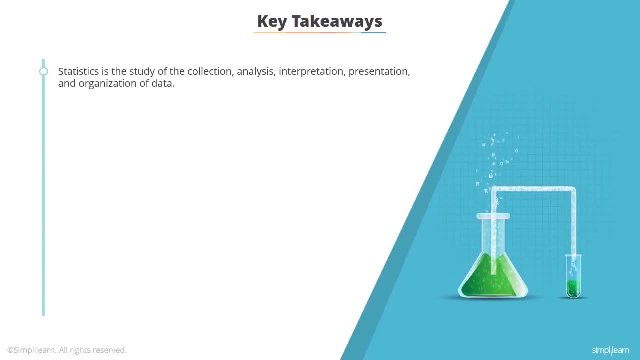 Statistics is the study of the collection, analysis, interpretation, presentation and organization of data. Statistical analysis is more reliable, as it is based on numbers and scientific analysis, when compared to non-statistical analysis. Descriptive and inferential are the two major categories of statistics. 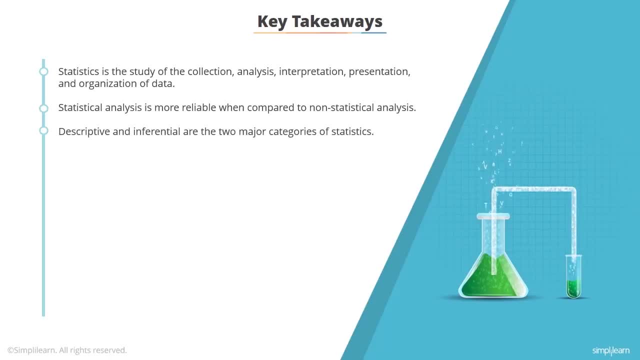 Descriptive takes into account all the members of the population, while inferential uses only a sample. Mean, median and mode are measures of central tendency, while variance and standard deviation measure the spread of data. The spread of distribution is called dispersion and is graphically represented by a histogram and a bell curve. 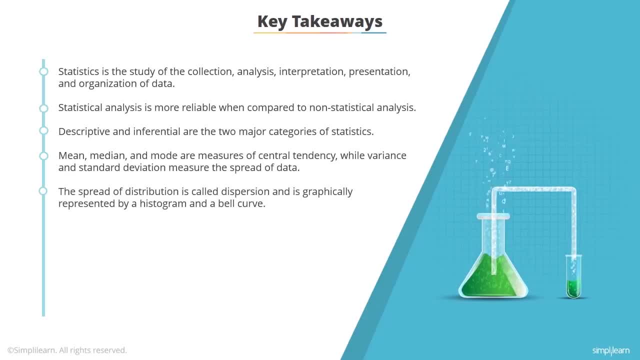 The shape of the dispersion is represented as left skewed, right skewed and kurtosis. Hypothesis testing is an inferential statistical technique that is useful for forecasting future patterns. Chi-square test is a hypothesis test that compares observed distribution to an expected distribution.